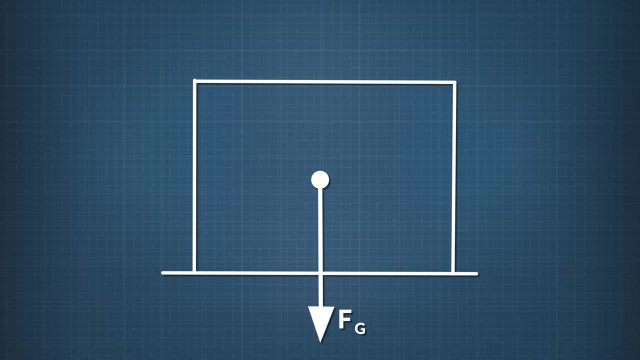 strong as gravity. We draw an arrow, starting at the center dot and pointing up equal in length with the gravity vector. We know it is equal in length because our box is at rest. The force acting up on the box equals the force acting down. We then will put a hash on each line to show. 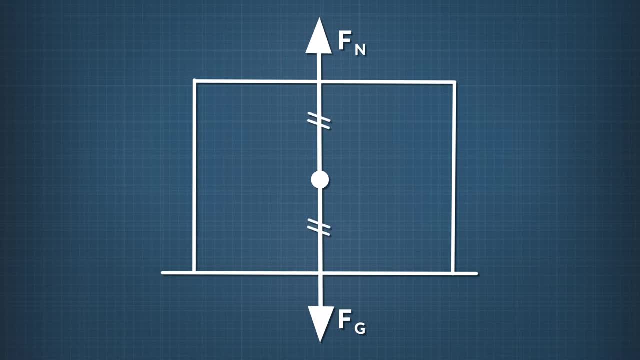 that gravity is acting down. Now what forces are acting on the shoebox? The force acting up on the that? they are equal. The free body diagram is now complete. There are two forces acting on the shoebox: gravity and normal force. Each is as strong as the other. 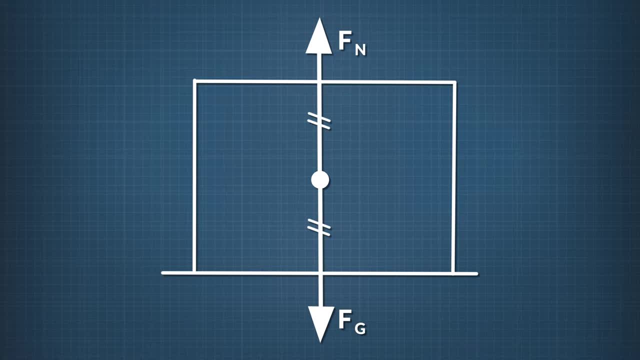 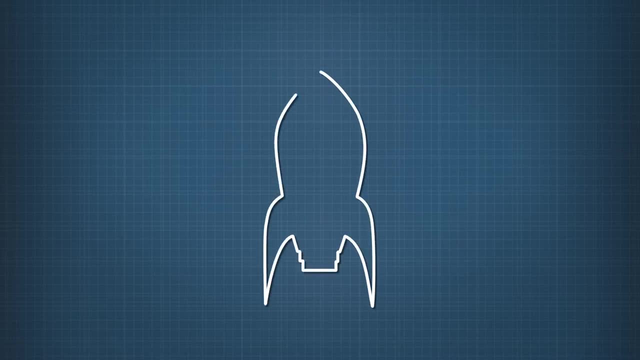 They cancel each other out and the box doesn't move. Now let's try an example where the object is in motion. After building a model rocket, you launch the rocket and watch it turn sideways while the fuel is still burning At that moment, with the rocket pointing horizontally. 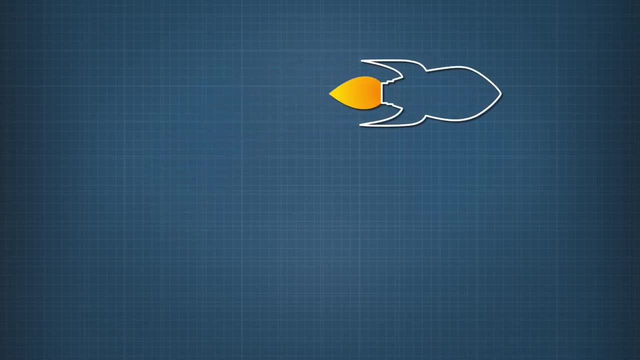 and the engine pushing it forward. what are the forces on the rocket? In what direction? up down, forward, backward, is it accelerating? We start with a sketch of the rocket outline and place a dot at its center of mass. What forces are acting on the rocket? 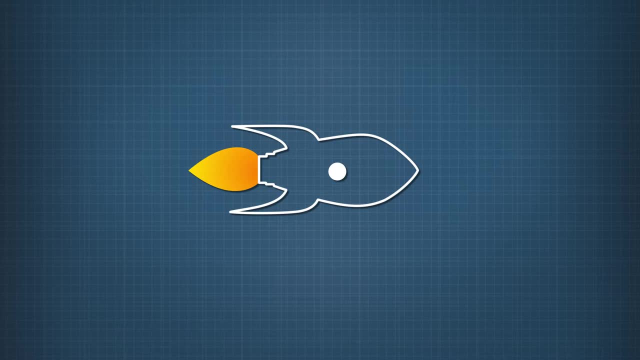 Gravity. We draw a downward arrow and label it F sub G. The thrust from the rocket engine is pushing the rocket forward. so we draw a forward facing arrow and label it F sub thrust. Are there any other forces involved? There is one more. 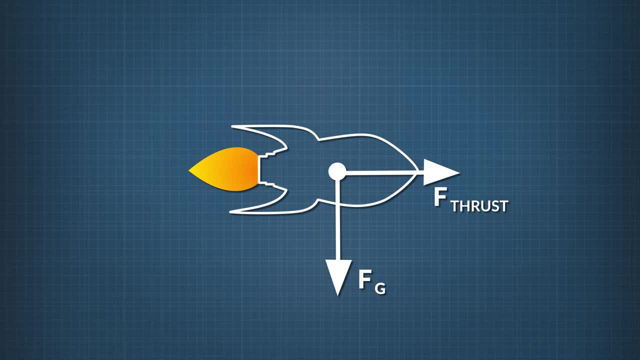 the resistance of the air to the rocket's motion. Air resistance is caused by friction and points opposite the rocket's motion. So we draw one last arrow in our diagram facing backward and label it F, sub F. for friction The air resistance is not as strong. 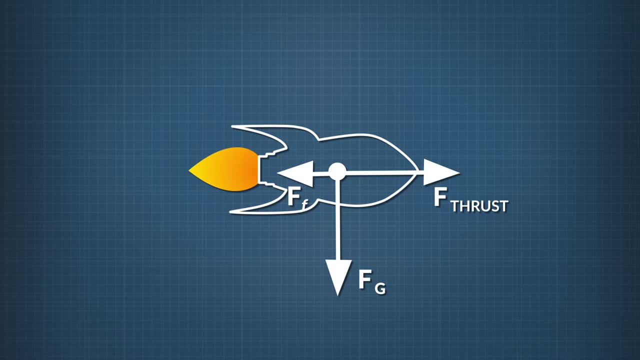 as the force of the rocket thrust. That means the arrow we draw for the friction force is shorter than F sub thrust. Using our completed free body diagram, we know that the forces acting on the rocket are gravity, engine thrust and air resistance or friction. 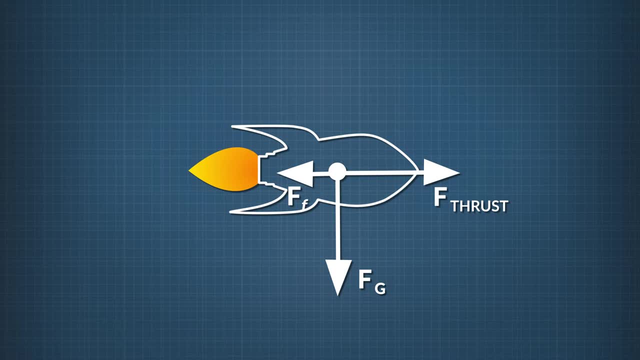 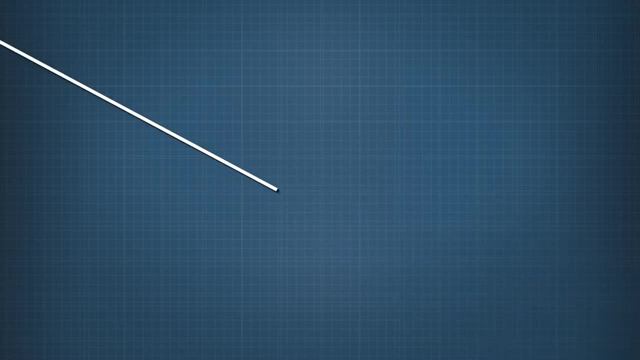 We also know the rocket is accelerating down because of gravity and forward because the thrust force is stronger than friction. For our last example, let's look at an object accelerating at an angle. You set a wooden block on a steep ramp and the block starts to slide down the ramp. 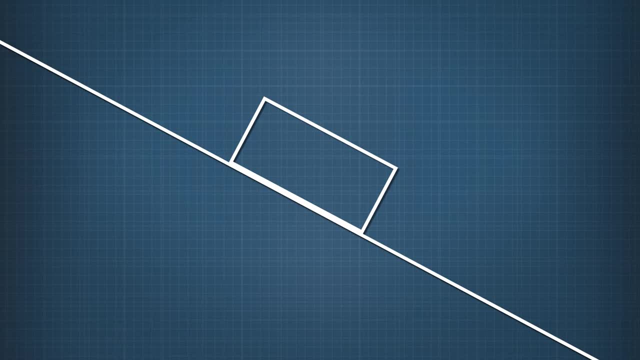 What forces are acting on the block and in what direction is the net force? Following our method, we first draw an outline of the block and put a dot in the center of it. Now for the forces involved. We know gravity pulls the block down. 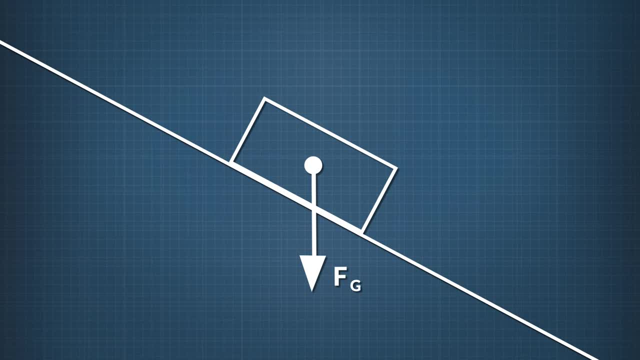 We draw that arrow in first and label it F sub G. What other forces act on the block? There's the normal force, but which way does it point? Remember, the normal force always points perpendicular to the surface exerting the force. In our case, that's the ramp. 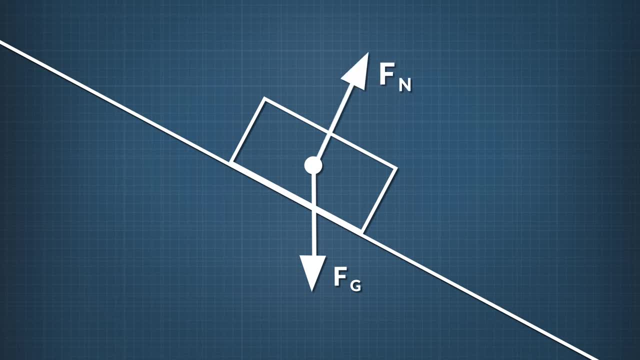 which pushes the block away from its surface. So the normal force points like this: What other force is acting on the block while it slides? If you said friction, that's the force acting on the block while it slides. If you said friction, that's the force acting on the block. 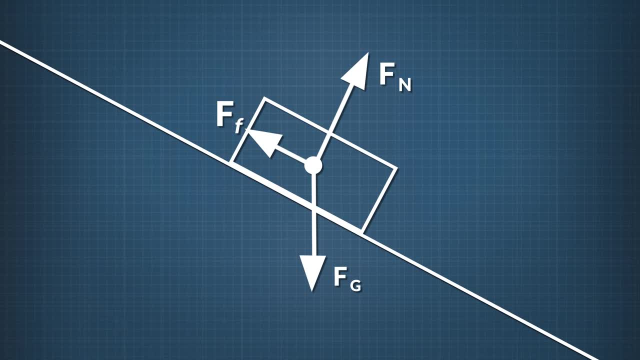 You're right. The force of friction acts parallel to the ramp surface and points opposite the motion of the block. It looks like this and is labeled F, sub F. Are there any other forces? No, The only forces acting on the block are gravity. 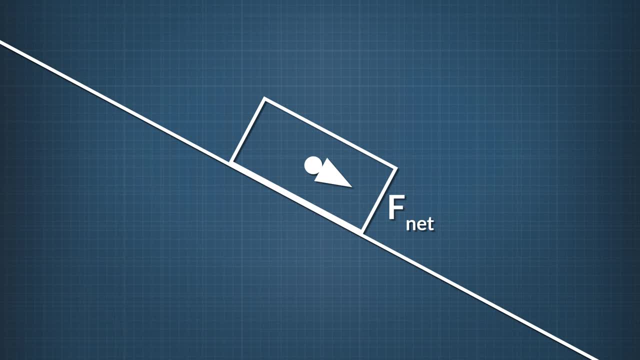 the normal force and friction. Combining these forces adds up to an arrow pointing down the ramp. The component of the force of gravity pointing down the ramp is stronger than the friction force and the block speeds up down the slope. That's a closer look at free body diagrams. 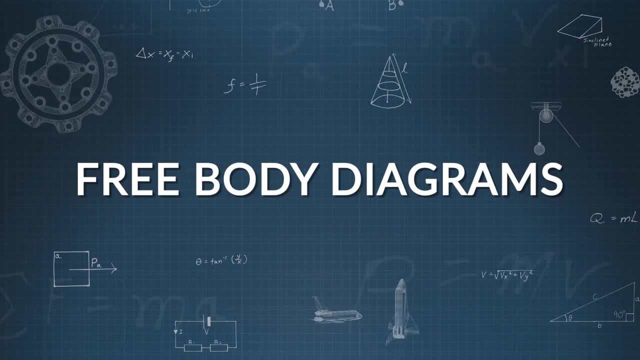 For more physics in motion, go to our homepage, where the entire series is available to you.